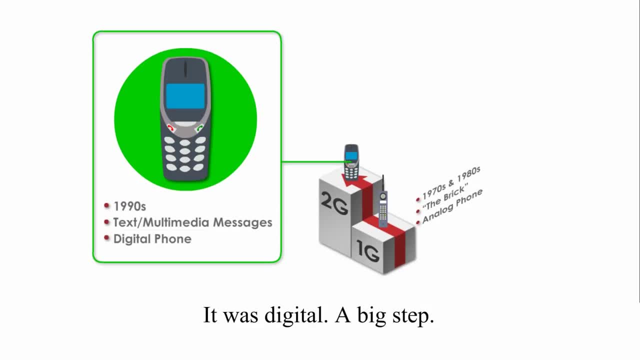 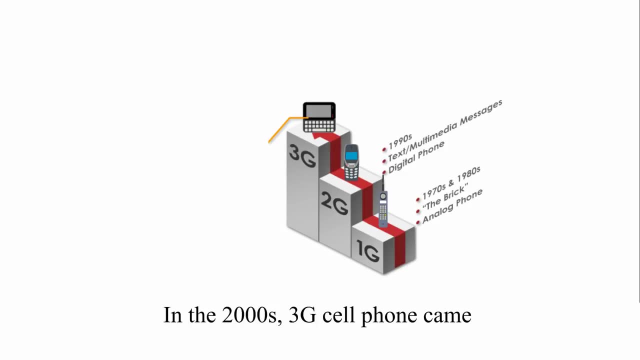 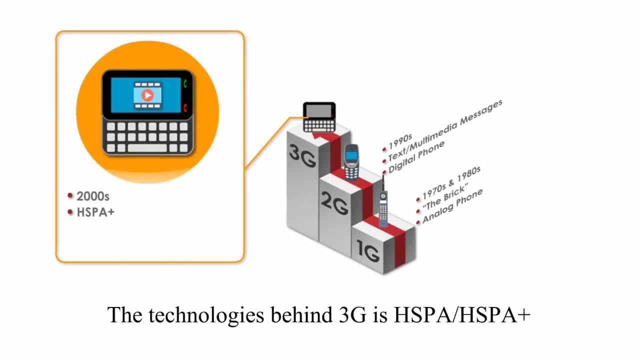 and you can even send a smiling face. It was digital- a big step. In the 2000s. 3G cell phones came with the Internet browser. The technologies behind 3G is HSPA or HSPA+. 3G used MIMO, multiple input, multiple output. 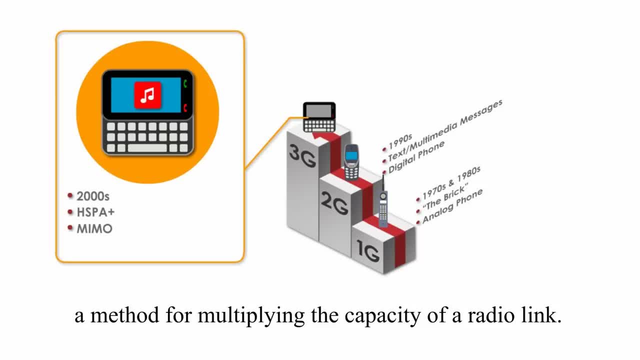 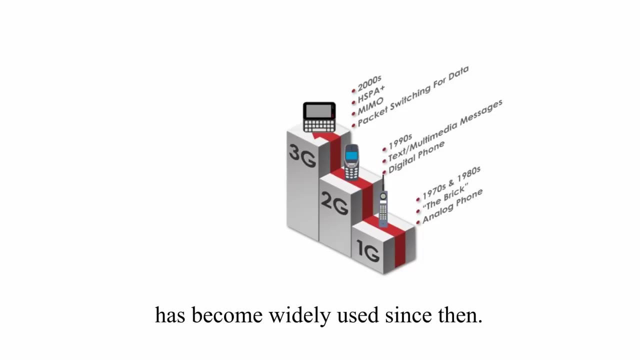 a method for multiplying the capability of radio link In data transmission. package switching method is used for 3G. Besides, the generation terminology has become widely used since then. In the 2010s, 4G cell phones came to dominate the market. 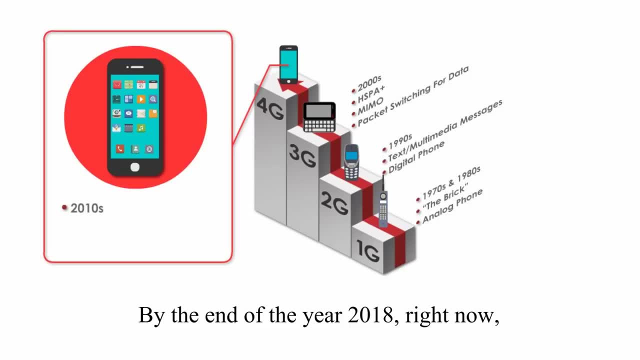 By the end of the year 2018. right now, pretty much everyone except grandma, grandpa is using 4G cell phones. Behind 4G are the internet. There are LTE, long-term evolution or WiMAX. 4G uses IP and package switching just like computers. 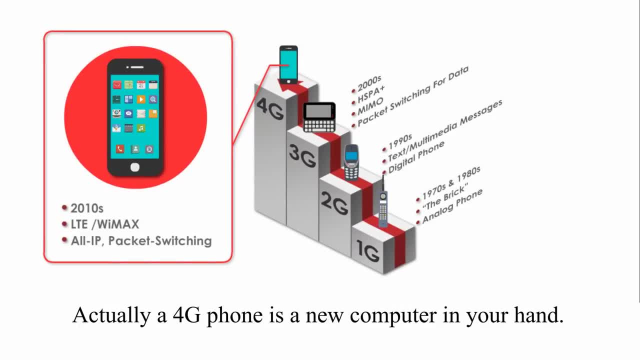 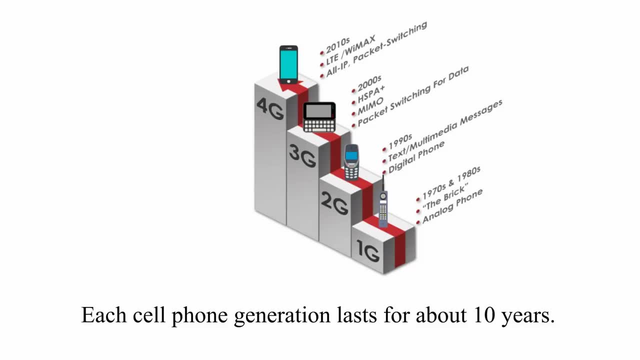 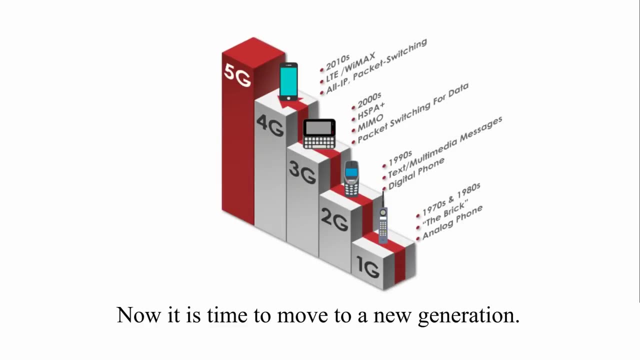 Actually, 4G phone is new computer in your hand. At this point, you might see the pattern. Each cellular phone generation lasts for about 10 years. Now is time to move to a new generation. The 2020s will be a 5G era. 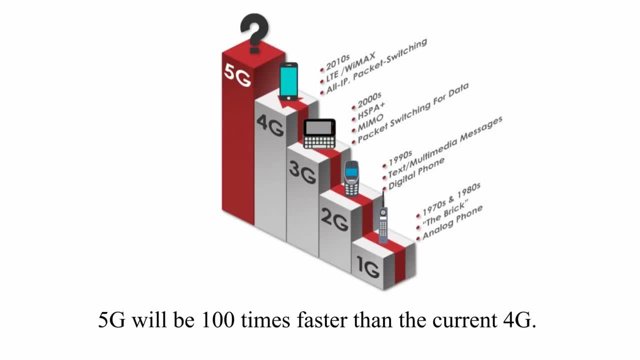 It is said that 5G will be 100 times faster than the current 4G, And the downlink maximum throughput can offer over 10 to 20 Gbps, which means you can download two to three high-definition DVD movies just in one second. 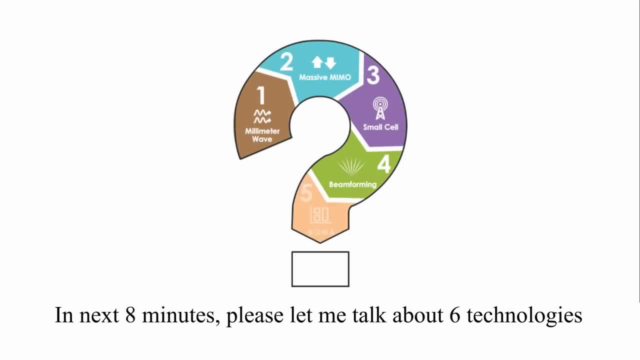 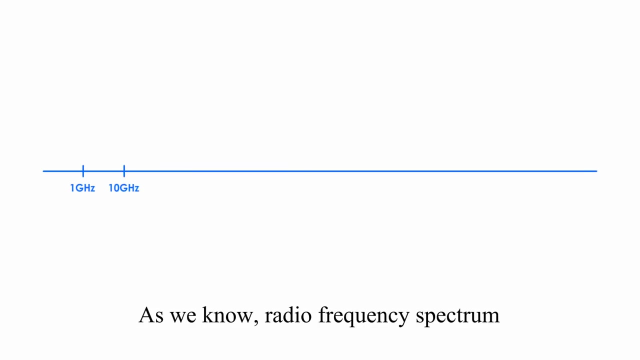 What makes 5G so exciting. In next eight minutes, please let me talk about six technologies, among many others, possibly used for 5G cellular network. 1. 5G will use new radio called millimeter wave, As we know. radio frequency spectrum from 1 GHz to 6 GHz. 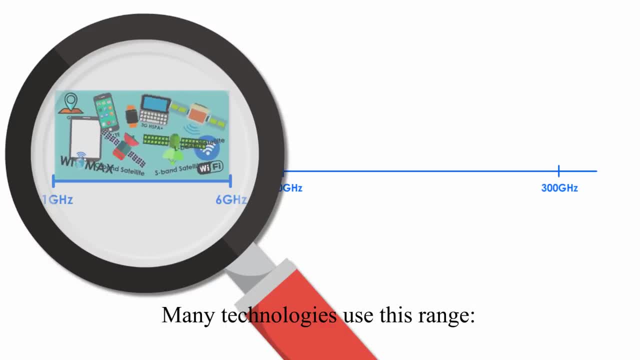 is very crowded. Many technologies use this range, such as GPS, WiMAX, Wi-Fi, 4G, 3G, L-band satellite, S-band and C-band satellite, etc. The spectrum range from 30 GHz to 300 GHz. 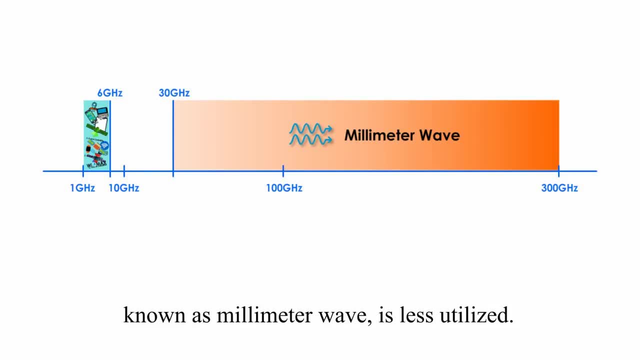 known as millimeter wave, is less utilized, is a new territory. Thus, the range from 24 GHz to 100 GHz is proposed for 5G. The millimeter wave has at least three advantages: 1. It is a new and less used band, as we mentioned before. 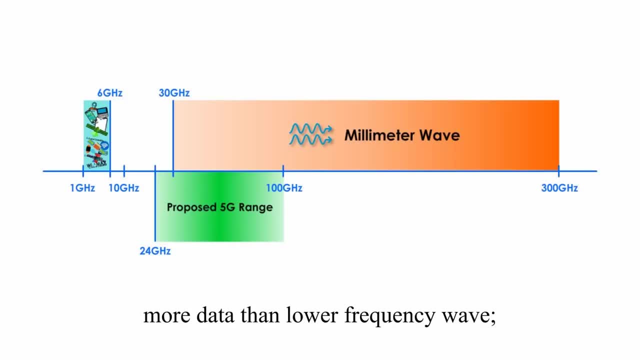 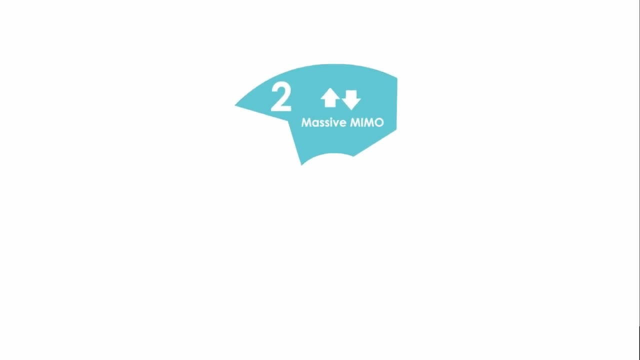 2. Higher frequency wave carries much more data than lower frequency wave. And the third advantage is millimeter wave makes possible to have massive MIMO antenna, which is the second 5G technology. The relationship between the wave frequency and antenna size: 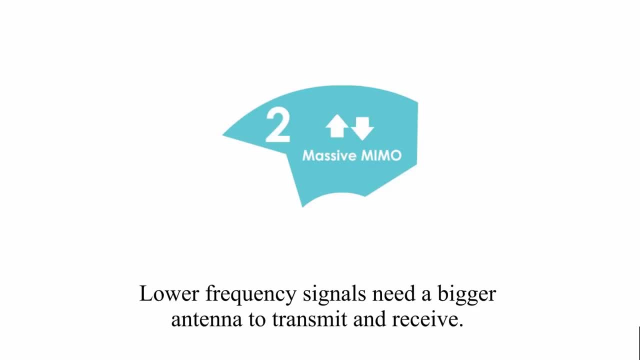 is inversely proportional, which means lower frequency signals need a bigger antenna to transmit and receive, while the higher frequency signals can work well with the smaller size antenna. The higher frequency wave we use, the smaller antenna we can get. Thus millimeter wave makes it possible. 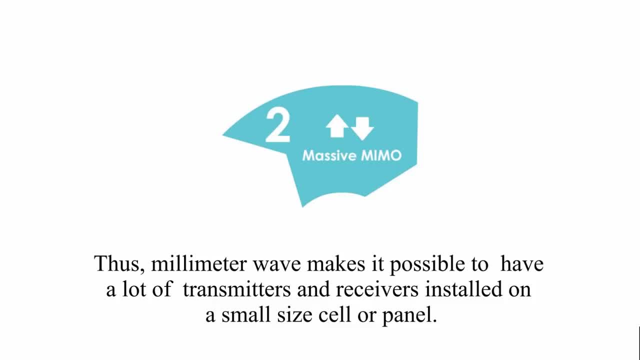 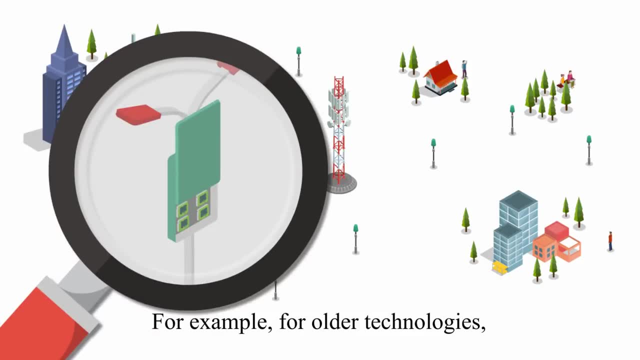 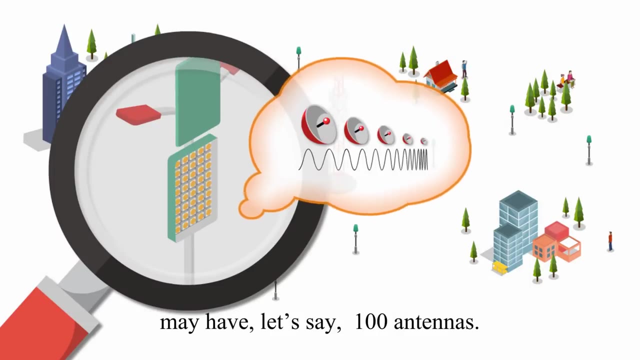 to have a lot of transmitters and receivers installed on a small size cell or panel. For example, for older technologies one cell can have 10 antennas, but for 5G the same cell may have, let's say, 100 antennas. 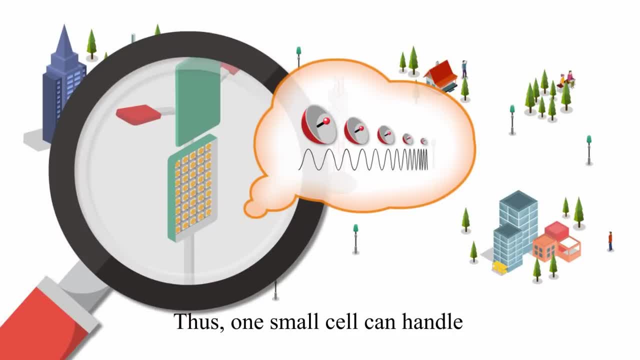 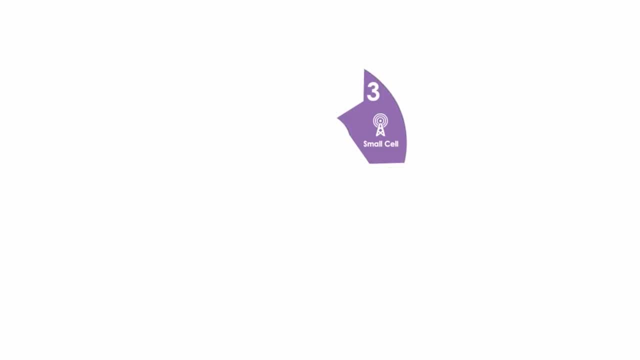 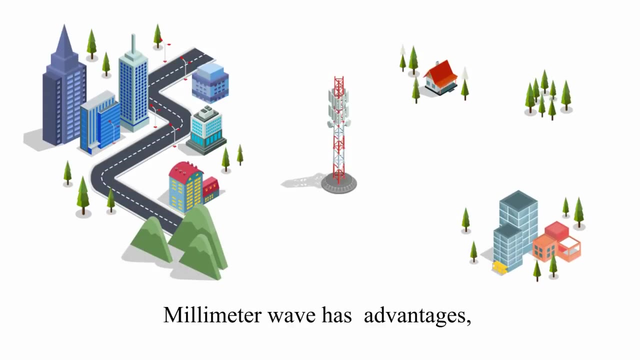 Thus one small cell can handle many more users at the same time. The third technology is also related to millimeter wave. Millimeter wave has advantages, as we mentioned before, but it has some disadvantages too. For example, higher frequency signals will have more collisions. 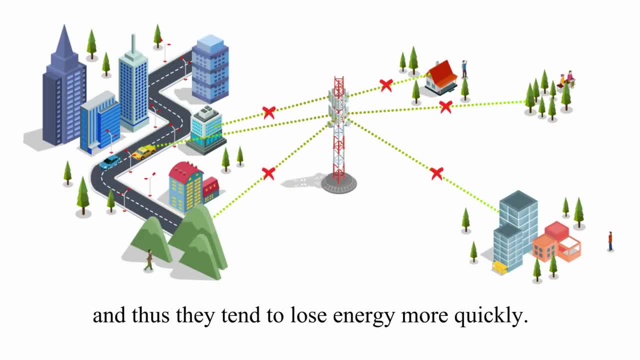 with obstacles in the air, and thus they tend to lose energy more quickly. Therefore, millimeter wave signals cover shorter distances. They are also easily blocked by buildings or trees. To solve these problems, small cell stations are needed to fill in coverage gaps. 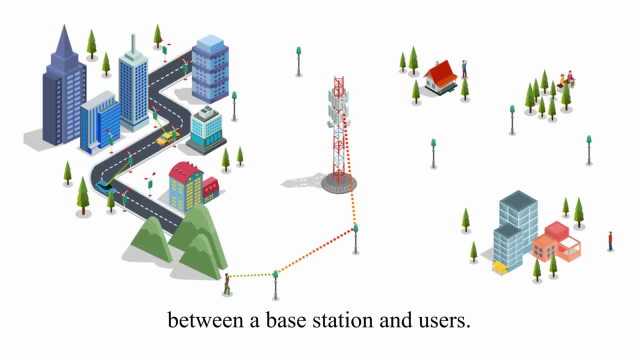 They are also used to fill in coverage gaps between the base station and the users. Each cell station covers a small area. The number of small cell stations and the distance between them depends on the population at that location, In a highly populous district, for example. 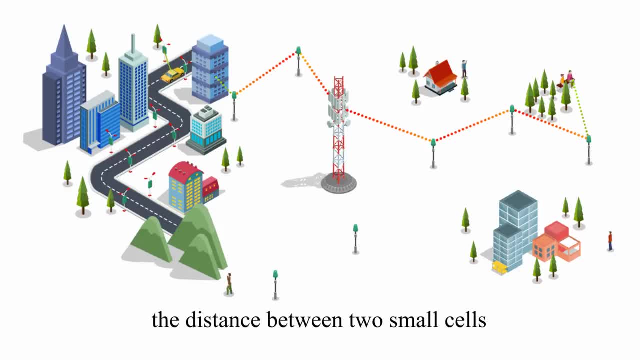 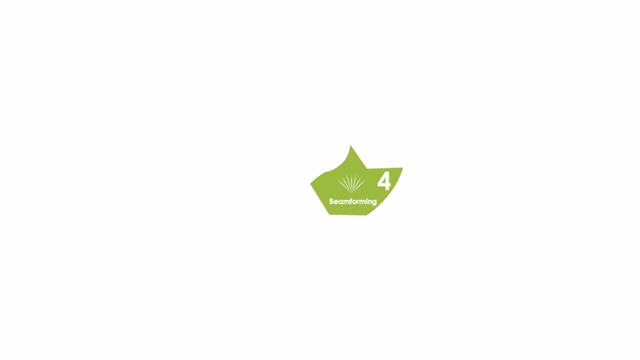 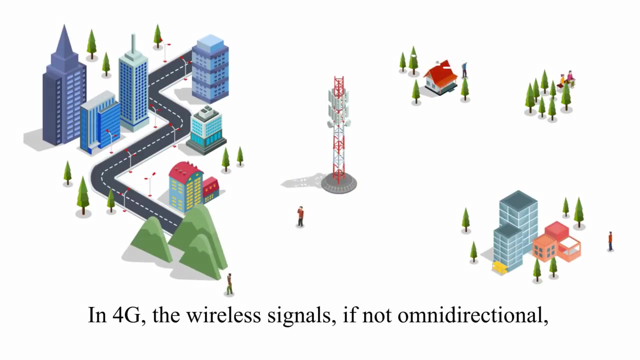 the distance between two small cells could vary from 10 to 100 meters- 100 meters. In the near future you might see such small cells everywhere in your neighborhood. The fourth new technology is called beamforming. In 4G, the wireless signals, if not omnidirectional. 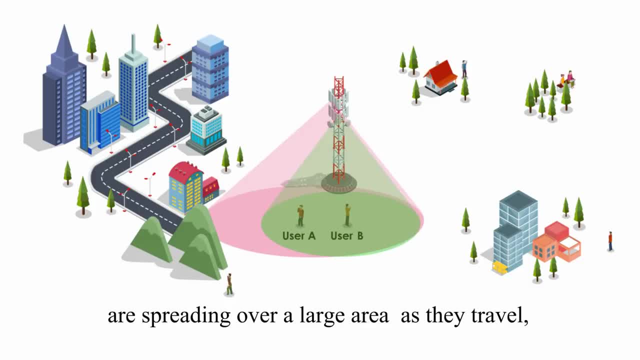 are spreading over a large area as they travel. Thus, signals tend to lose energy more quickly. To make things worse, different users might interfere with each other if they are standing close. Beamforming makes the transmission between the users and the base or cell stations. 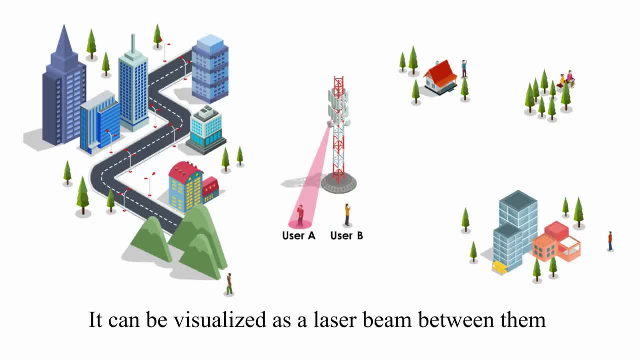 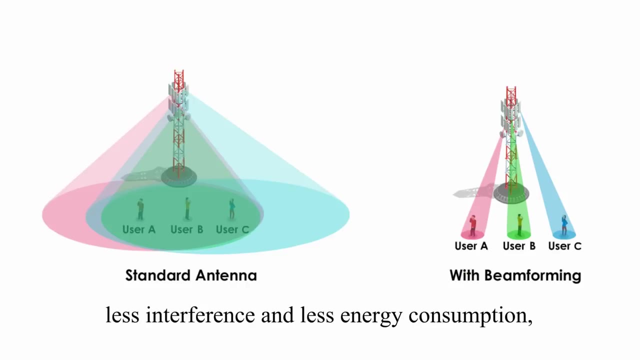 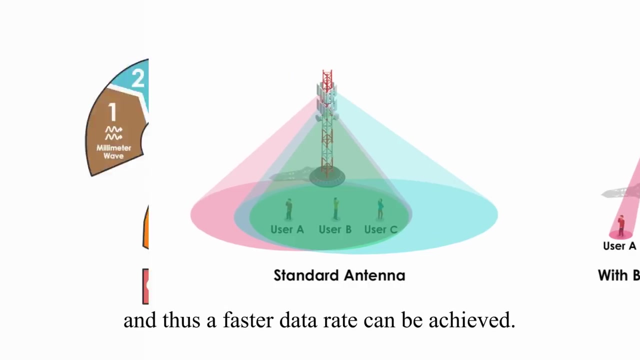 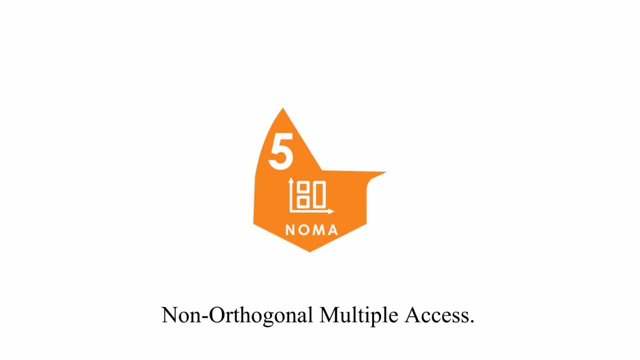 more directional. It can be visualized as a laser beam between them, so that signals seem like traveling along an invisible cable. The high density of beamforming leads to less interference and less energy consumption, and thus a fast data rate can be achieved. The fifth technology is NOMA. In previous generations, 1G through. 3G. the beamforming technology was used to measure the density of the beam. In the past, the beamforming technology was used to measure the density of the beam In the past. the. The fifth technology is NOMA. In the past, the beamforming technology was used to measure the. 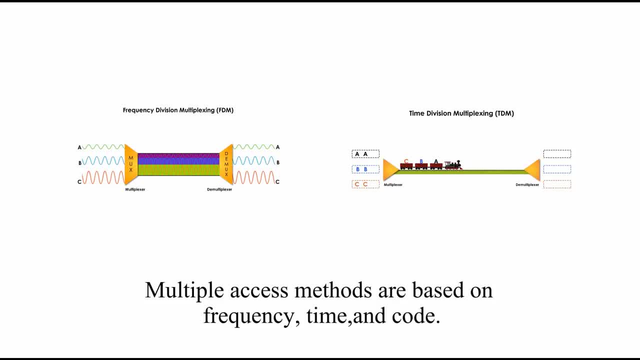 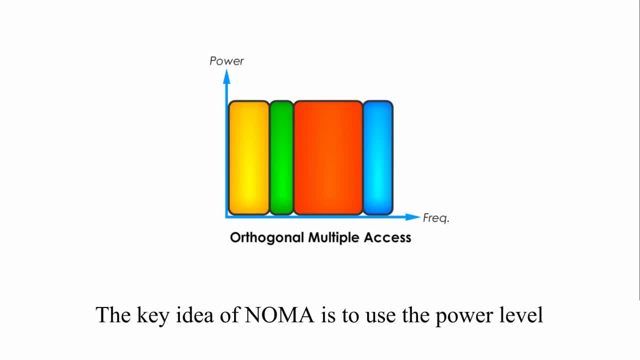 density of the beam. The beamforming technology was used to measure the density of the beam, For example, in a 4G multiple access methods are based on frequency, time and code. In 4G, orthogonal multiple access is used. The key idea of NOMA is to use the power level. 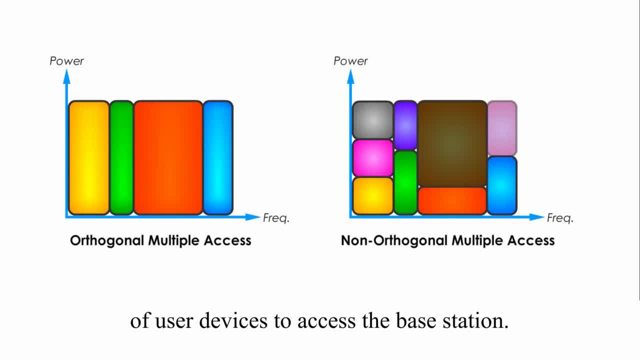 of user devices to access the base station. The new multiple access method would allow different signals share the same channel simultaneously, but NOMA provides a high summary than orthogonal method. These two access methods, orthogonal and non-orthogonal, would be two separate videos on my channel. Here I try to skip the details otherwise. 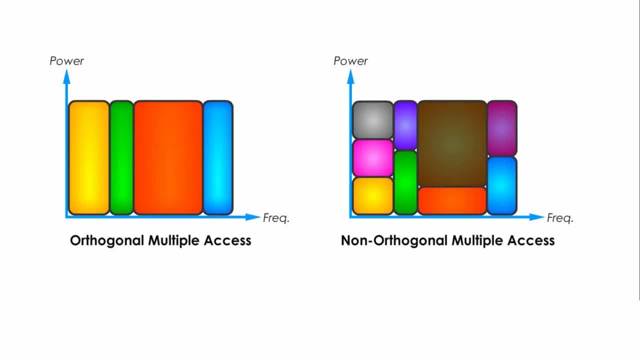 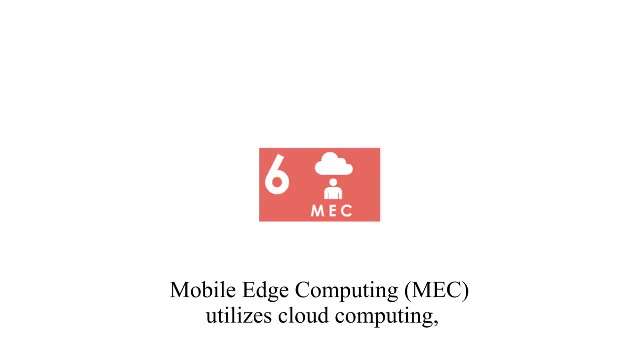 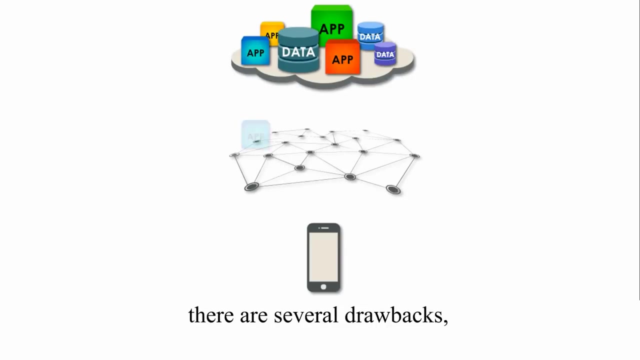 this video is already too long and too boring. Last but not least, mobile edge computing. Mobile edge computing, or MEC, utilizes cloud computing, but brings cloud computing closer to users. In normal cloud computing environment. there are several drawbacks, which include: one: cloud service could be far away from. 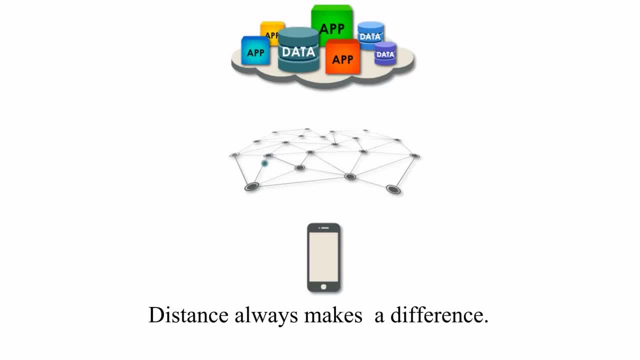 users physically. You know cloud service always makes difference. Longer distance would easily create latency. Two: many data and applications need downloading to users' devices. It would be too much burden to users' device, especially for the device with limited processing power and memory. 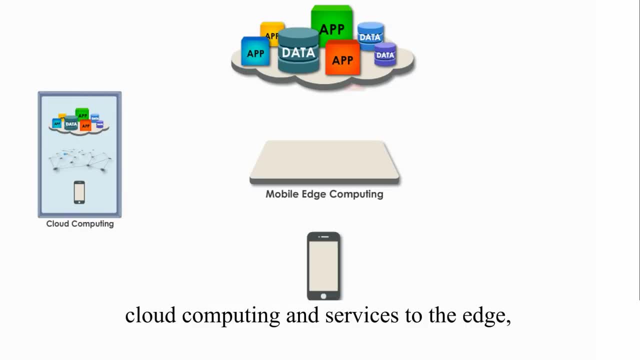 Mobile edge computing brings cloud computing and services to the edge, which is closer to the user. They are physically local to users. Intensive and latency-sensitive applications, like the augmented reality video conference, can be hosted at the edge of the network. Application splitting is another benefit. This would enable applications to be split. 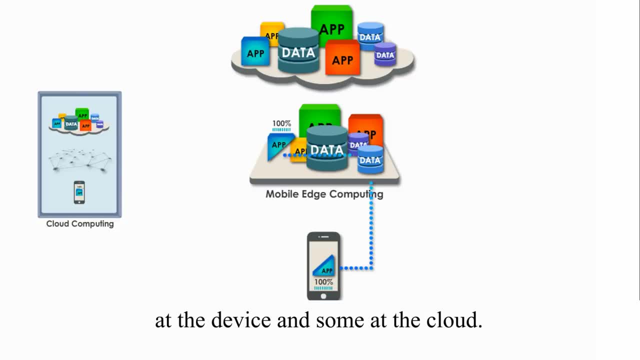 into small tasks, with some performed at the device's end. Here I list what model I have establishedindeós review – deep-up-correct to dogslimitingcomENGbe The animatedworth hologram by the features: clear: no focus focus output to be used as an. and some at the cloud. 5G would be driven by a lot of new technologies. On the other hand, 5G would push through other technologies to a new level, such as the Internet of Things, games, smart cities, smart homes, self-driving cars.